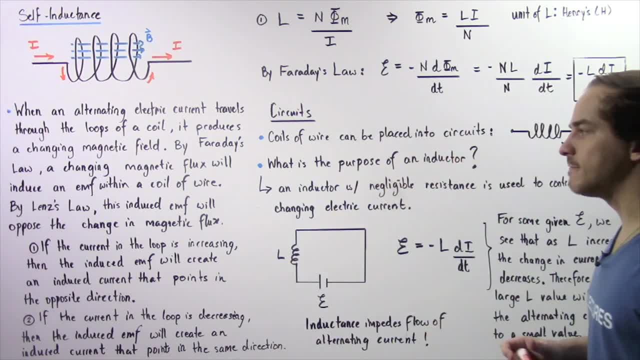 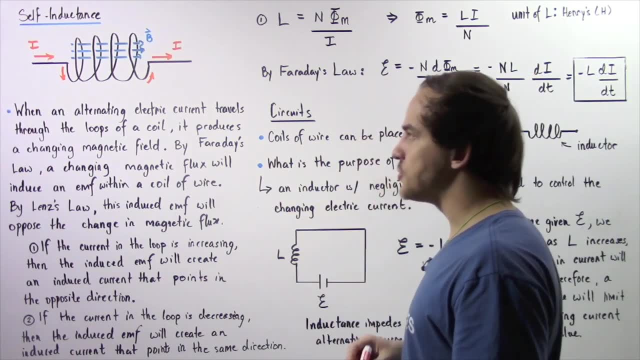 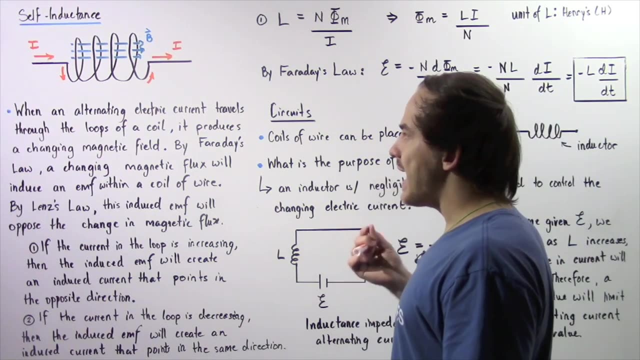 essentially oppose the change in magnetic flux. So we'll see exactly what that means in just a moment. First let's review what we just said. When an alternating electric current travels through the loops of coil, it produces a changing magnetic field. Now, because that magnetic field, 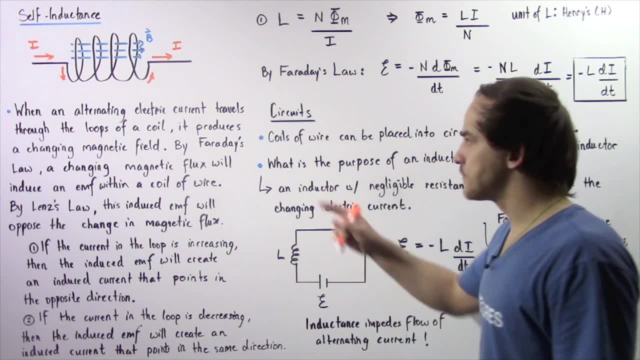 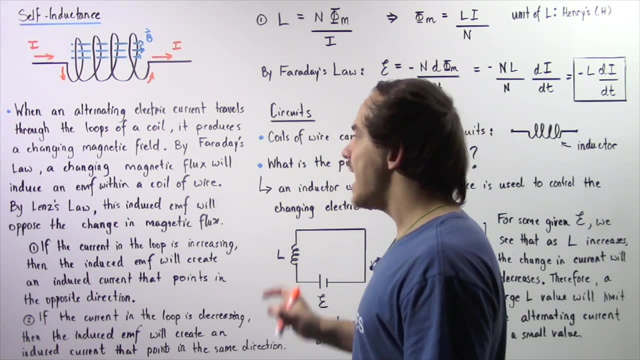 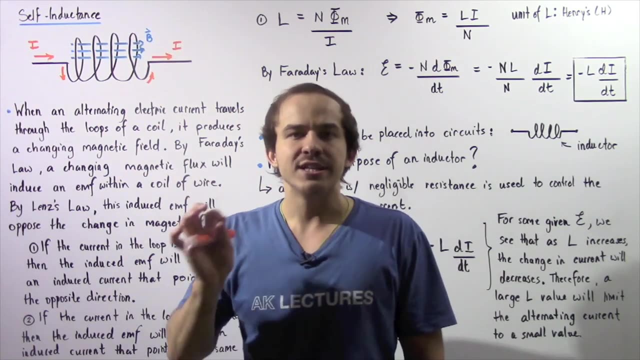 is changing, it will produce a changing magnetic field. Now, because that magnetic field is changing, that will change our magnetic flux. Now, by Faraday's law, a changing magnetic flux will induce an EMF within a coil of wire. So that will induce an EMF within this coil of wire and that induced EMF will. 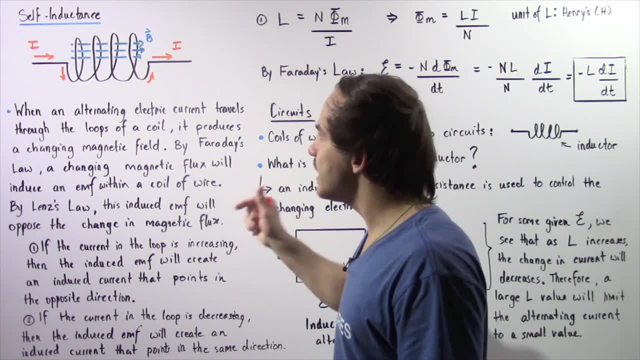 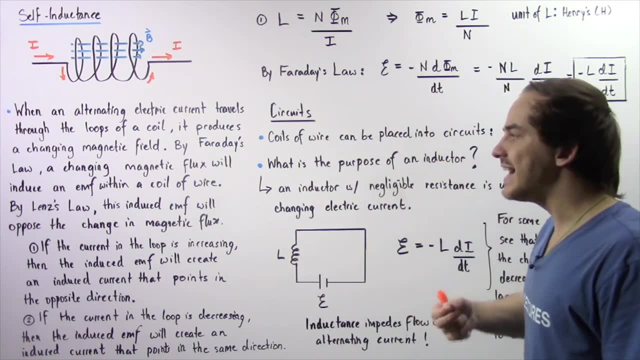 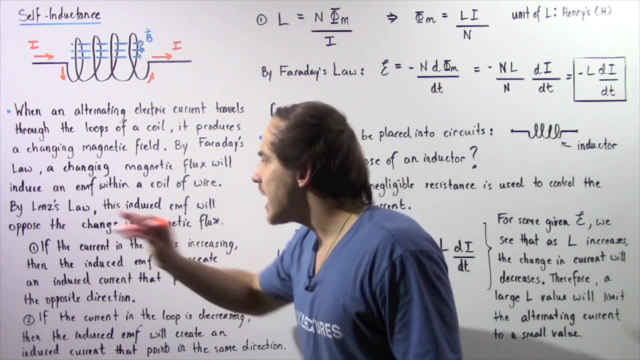 in turn induce an electric current within that loop of wire. Now, by Lenz's law, this induced EMF will create an electric current. Now, by Lenz's law, this induced EMF will create an electric current called the induced electric current. that will point in the direction that will oppose the change in 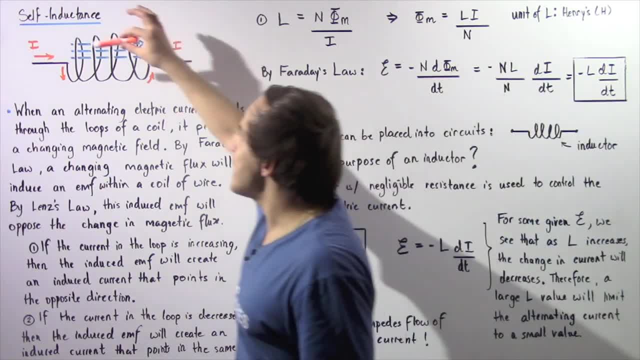 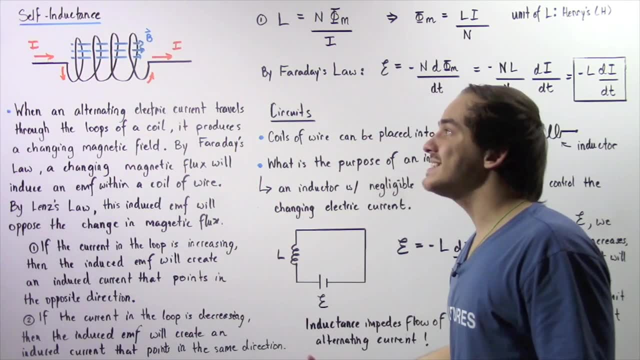 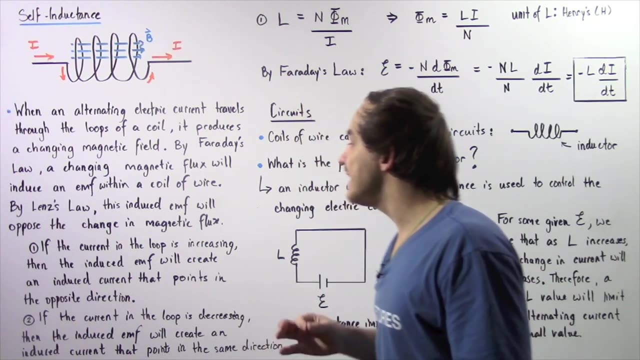 magnetic flux. So let's suppose that our electric current that is traveling through these loops of wire, that is an alternating current, is increasing at some given moment in time. Now, if the current that is traveling, given by I, is increasing, that basically means that the current is increasing. 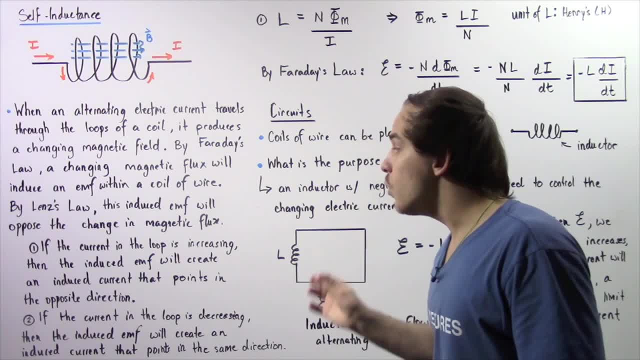 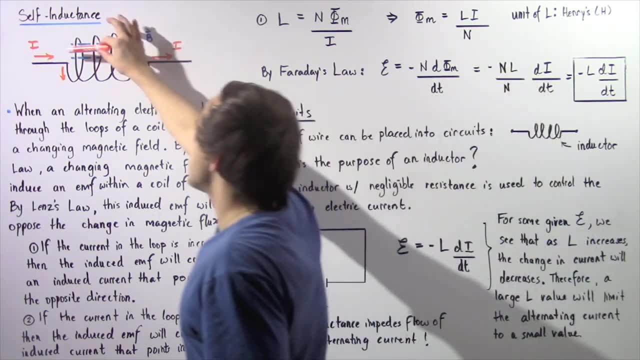 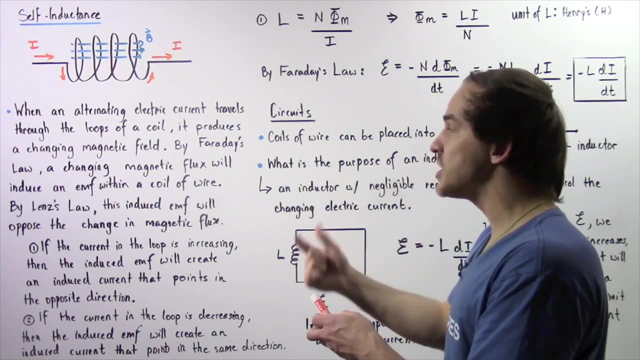 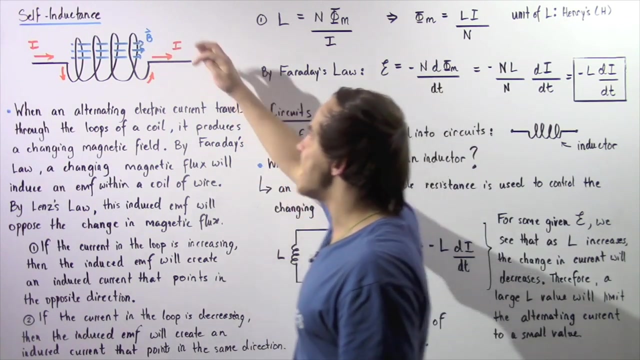 That basically means that the induced EMF will create an induced current that will point in the opposite direction of this electric current. and that's because our change in magnetic flux, our magnetic flux, is increasing, and so the induced electric current has to produce an induced magnetic field that points in the opposite direction of the magnetic field created by this. 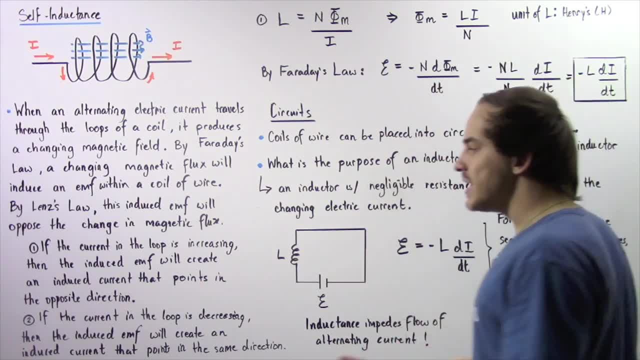 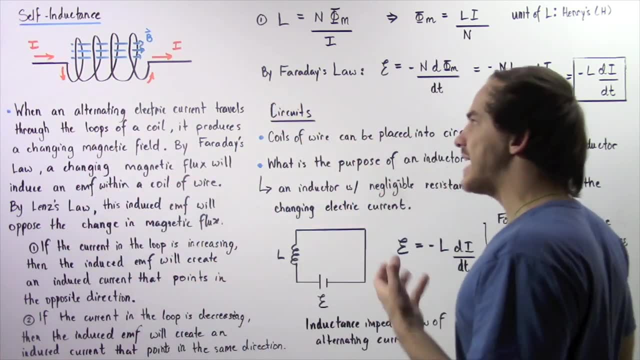 electric current Now by Faraday's law. a changing magnetic flux will induce an electric current that comes from Lenz's law. Now, on the other hand, if the electric current moving in the loop of wire is decreasing at some given moment in time, that basically means that our magnetic flux will. 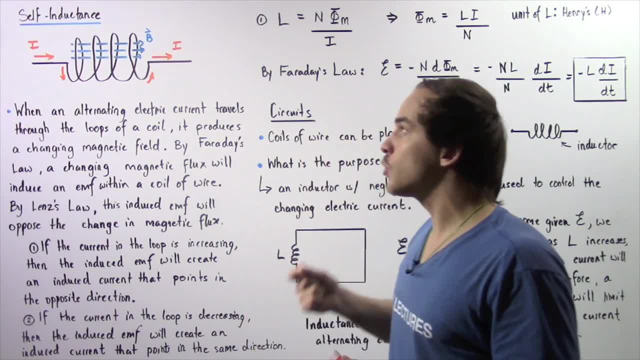 decrease, and so in our induced EMF we will create an induced electric current and that will create a magnetic field that will point in the same direction as this magnetic field and that implies that denotes that much function of the A-shape Further below. that is the aggression factor. privilege measuring A tension factor is when the Active Line force- x椎 Auto series automation cooked beneath itself 2020- andalts. constant frequency, causes force through the second e-y-y-x function into the second e-y-x function. 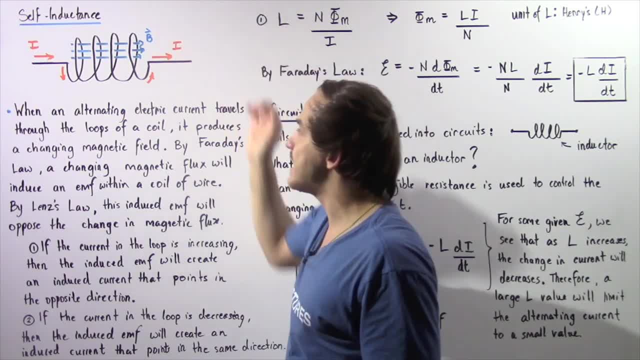 The parameter E-y-x function is by far-hand batteries, so the influence isure means that our magnetic flux is decreasing and if the e-m-f will around, it will delt. the electric current, Energy Principles point in the same direction as this magnetic field and that implies that the two electric 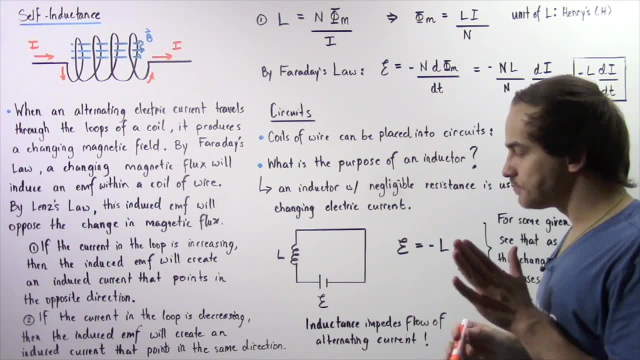 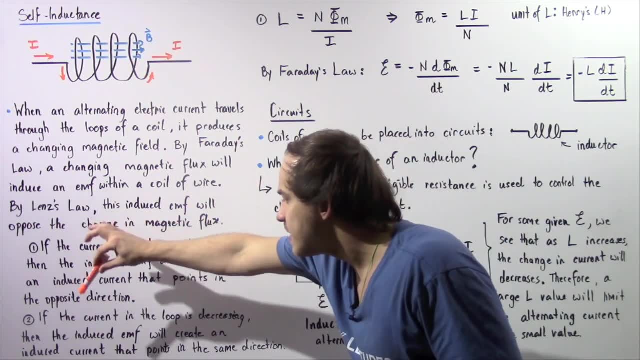 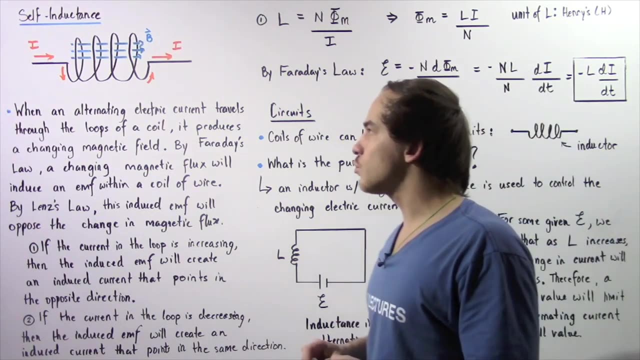 currents will point in the same exact direction. So, once again, if the current in the loop is decreasing at some given moment in time, then the induced EMF will create an induced electric current that points in the same direction as the initial alternating electric current. 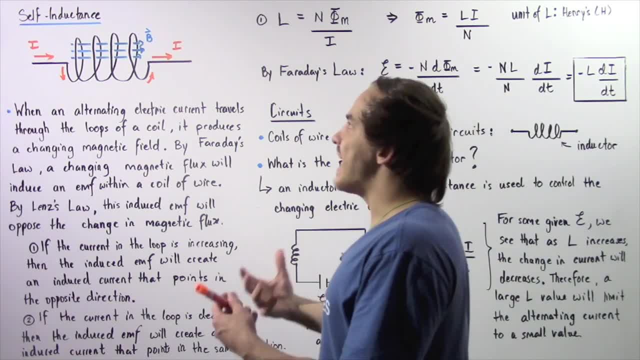 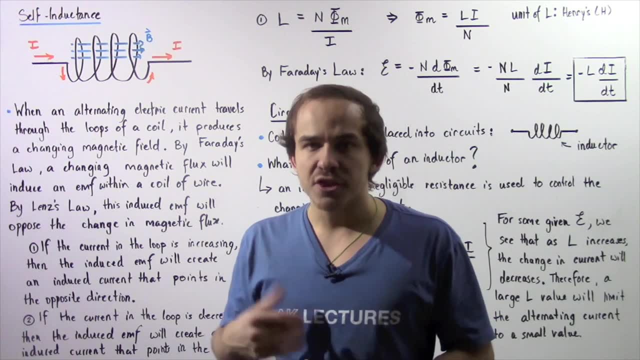 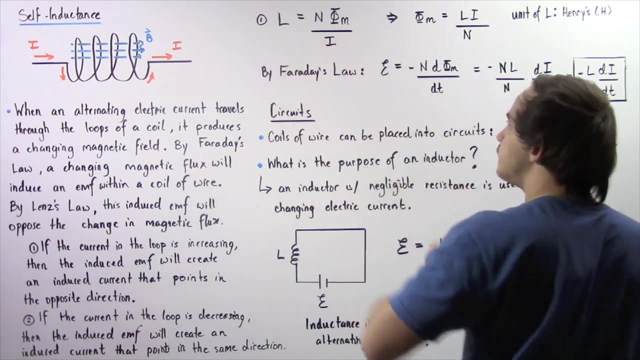 So this concept is known as self-inductance or simply inductance. Now let's actually define self-inductance mathematically. So in the same way that we were able to define mutual inductance, we can also define self-inductance. Self-inductance is given by uppercase L, So 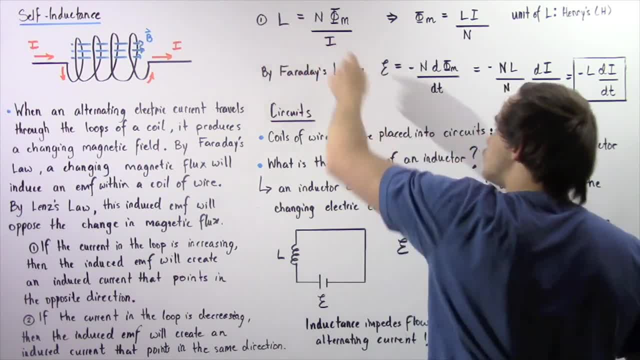 our self-inductance, or simply inductance, is equal to the product of the neutral electric current. So if the current in the loop is decreasing at some given moment in time, then the induced electric current will really create an induced electric current. 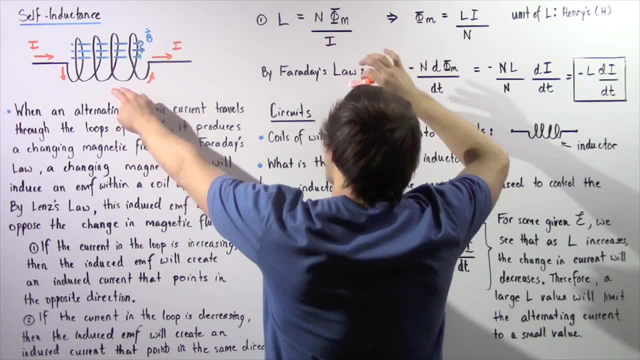 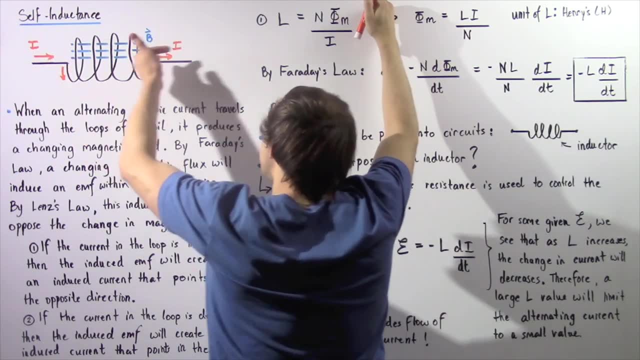 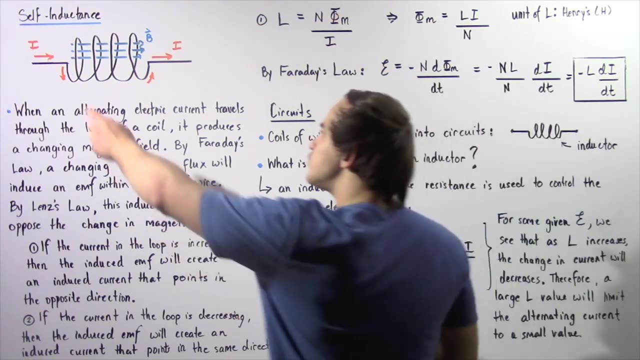 So, in order to learn this concept, let's actually have an injection in the loop where we'll find the distance which is: ay, it's not exactly a circle, it's the angle. So we'll just have to know what this distance is: The width at which the current is moving and the群ή مث past in. 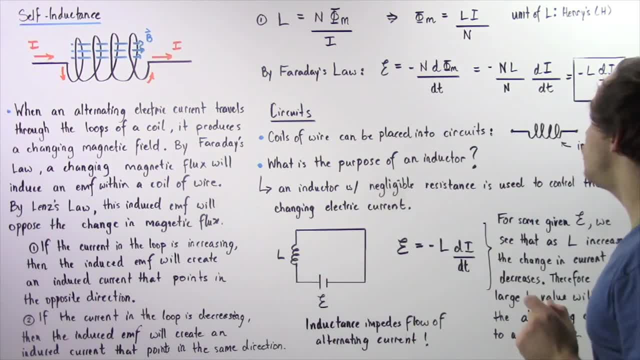 the loop will explain this through, Where we have a few rules in mind. if we have to build electric currents, that的 two är ripős. We are 아니야, or right When this is done with a Madame tastelaar on the electric current. we're actually delivering an electric current through the this wire By doing 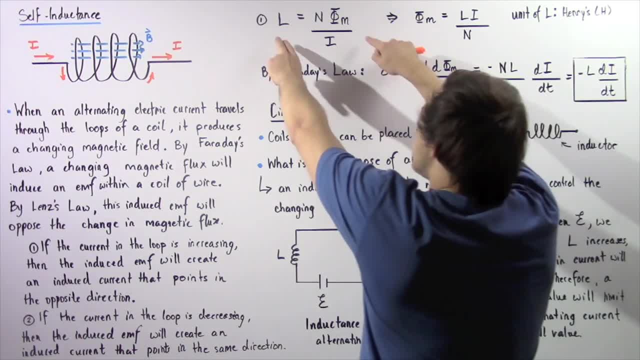 this we're giving itsembling with higher and higher power. Hah, Thanks to one. 행복 hay is. uh, we've got Mr filling the matrix, that bit he's pointing out in bold and your feeling, case H. Now, if we take this equation, we can rearrange it and solve for our magnetic flux. 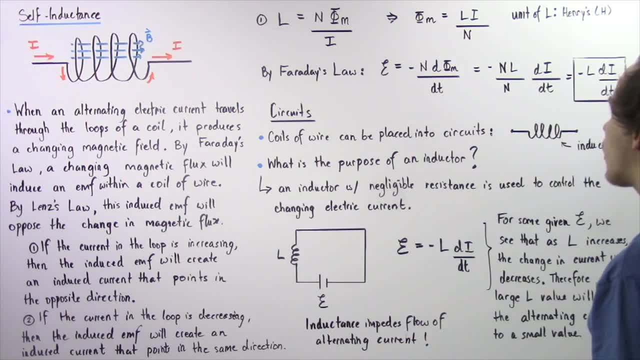 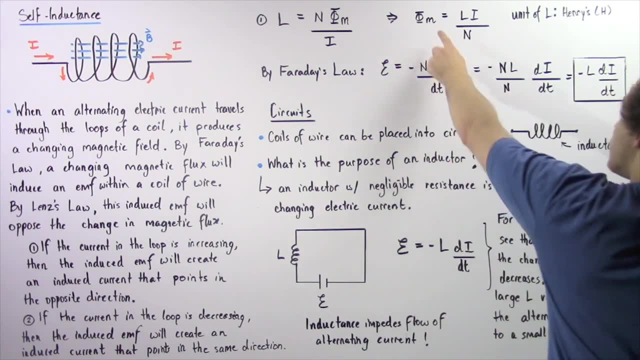 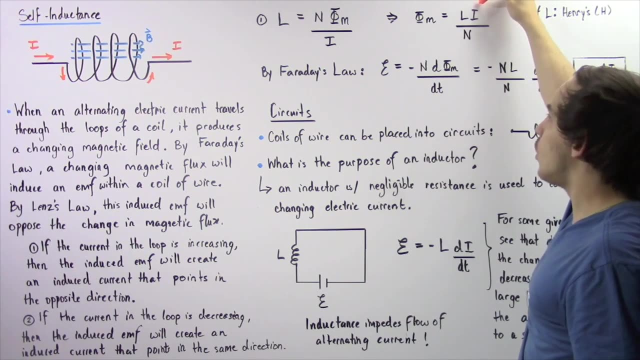 that exists within these loops of wire of our coil. So we see, if we bring the I and N to the left side, we get the following result: The magnetic flux within our coil of wire is equal to the product of our inductance, L multiplied by I, our current- divided by N. 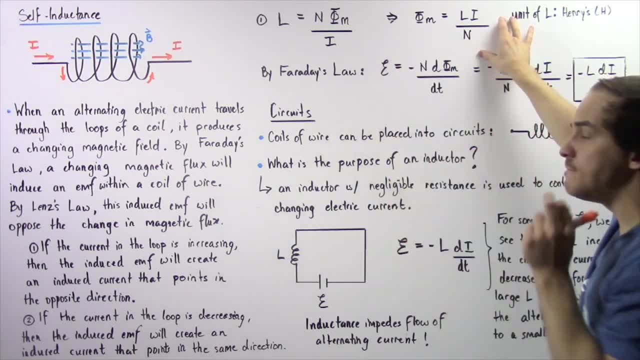 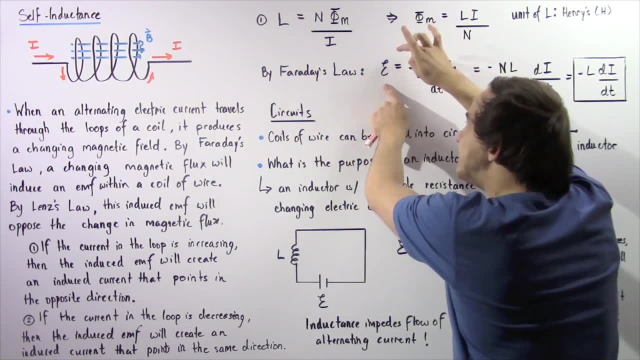 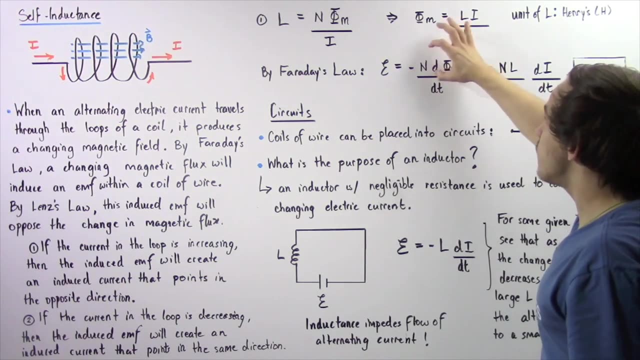 So now let's combine this equation with Faraday's law of electromagnetic induction. By Faraday's law, we know that our induced EMF within our coil is equal to the negative of the product of the number of loops given by N, multiplied by the derivative of our magnetic 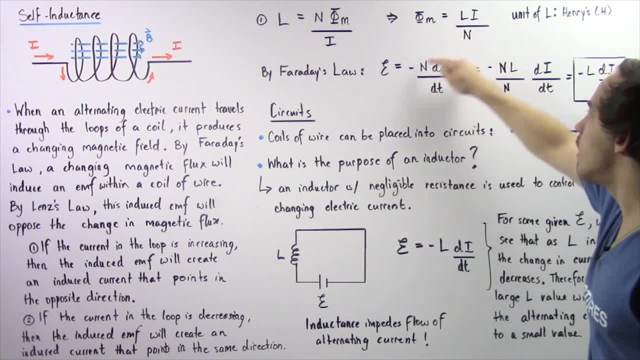 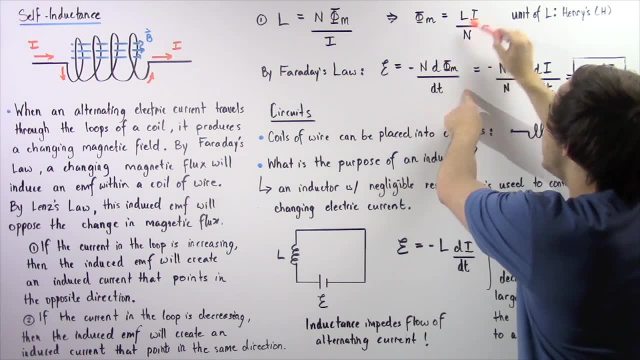 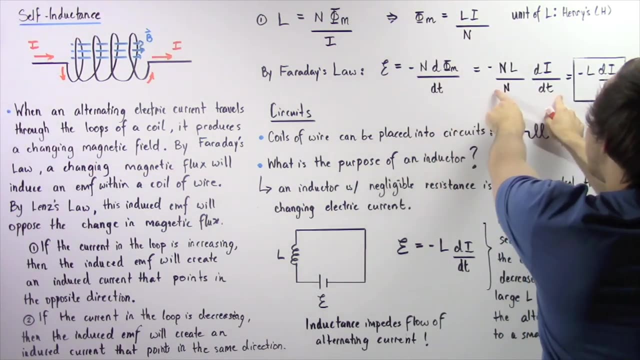 flux With respect to time. So the rate of change of our magnetic flux with respect to time. Now, from this equation we know that this quantity is equal to Li divided by N. So if we take that and plug it in, we get the following result: 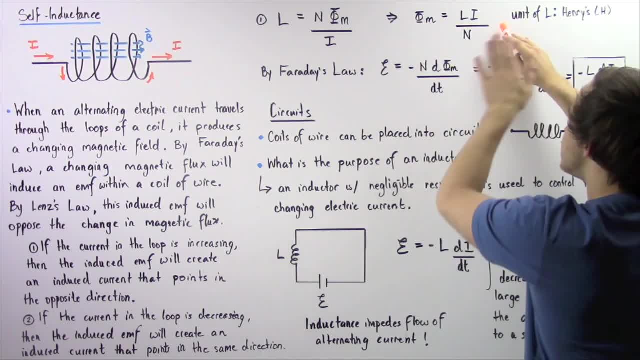 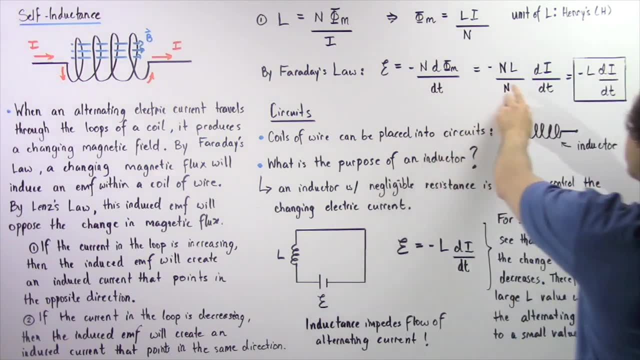 So we can take out our constants. L and N are both constants, We can take those out, and the I is the quantity that varies over time. So that becomes The following: So our induced EMF is equal to negative of the product NL divided by N multiplied by 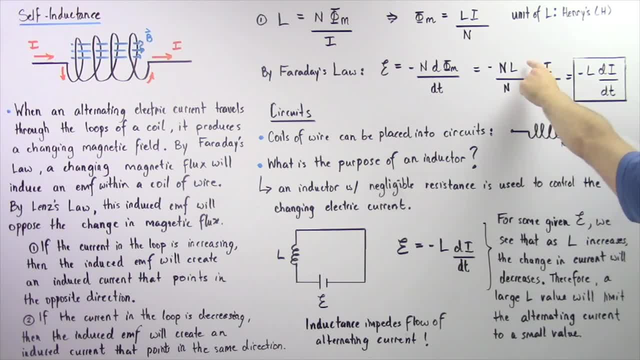 the derivative of our I with respect to T, So Di, Dt. Notice the N's appear on top and bottom. We can cancel these out and our equation becomes as follows: So this equation essentially gives us a relationship between our induced EMF and our inductance. 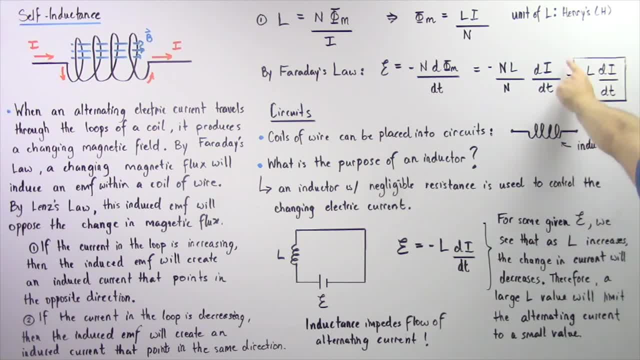 So now we can take out our constants: L and N are both constants. So now let's combine this equation with Faraday's law of electromagnetic induction, EMF and the rate of change of our electric current, So we see if our rate of change increases. 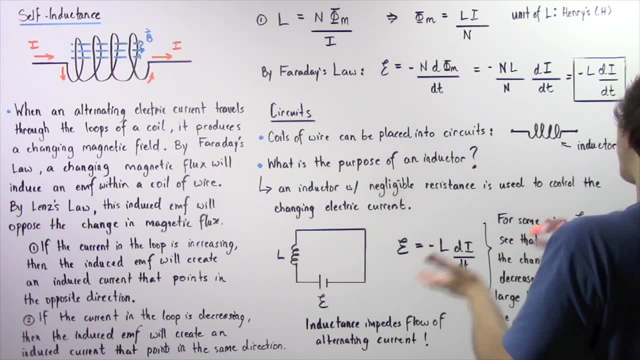 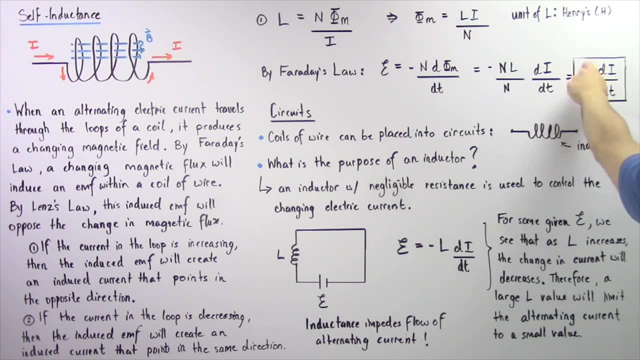 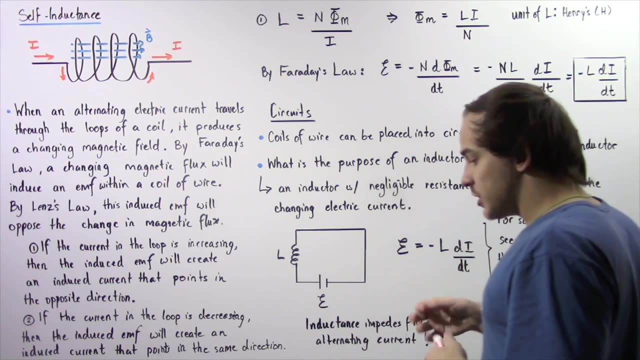 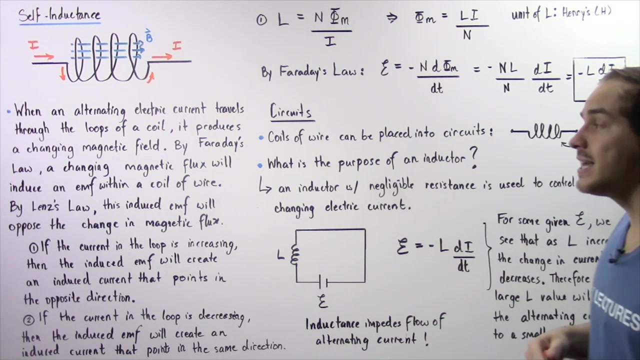 that will increase our EMF produced by that rate of change increase. So our EMF is equal to negative of our inductance, L multiplied by dI dt. So L is essentially a constant. but L depends on the type of coil that we are using. It depends on things like the shape, size and the distance. 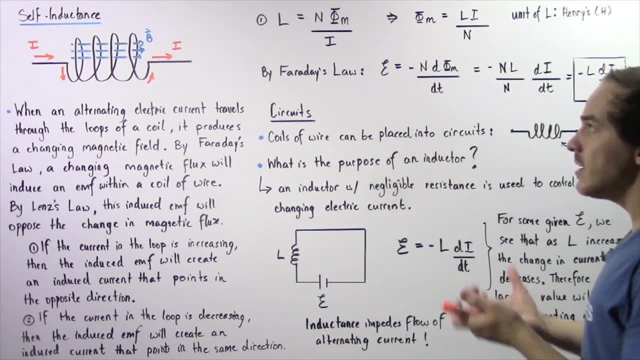 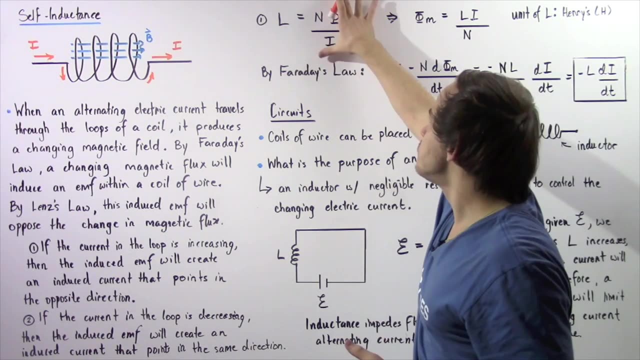 between our coils. So inductance are found inside circuits. So coils of wire can be placed into circuits, and these are known as inductors. And this particular inductor has an inductance given by L, given by this equation. Now, what exactly is the purpose? 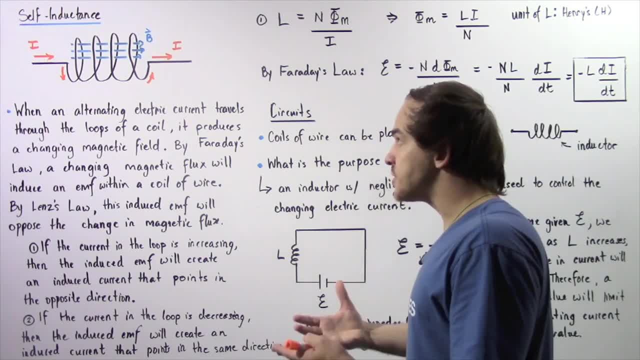 of the inductance. Well, the purpose of the inductance is that it is a function of the inductance, So inductance is a function of the inductance. So inductance is a function of the of an inductor. When we take an inductor, which is essentially a coil of wire, and place it inside, 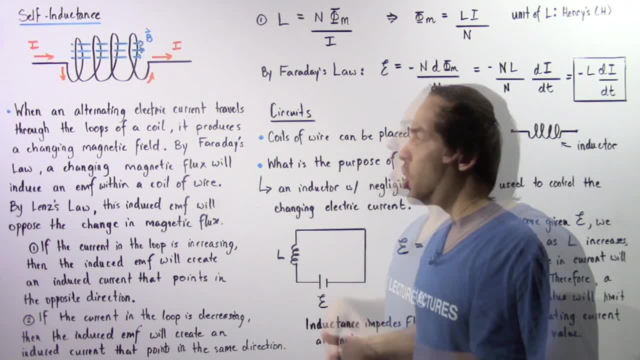 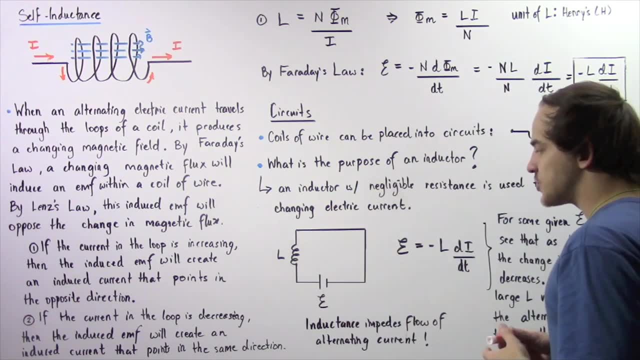 an electric circuit with some source of voltage. what purpose does that serve? So let's suppose we have the following electric circuit, So we have some type of voltage source and that creates an alternating electric current which travels through our electric circuit. So what is the 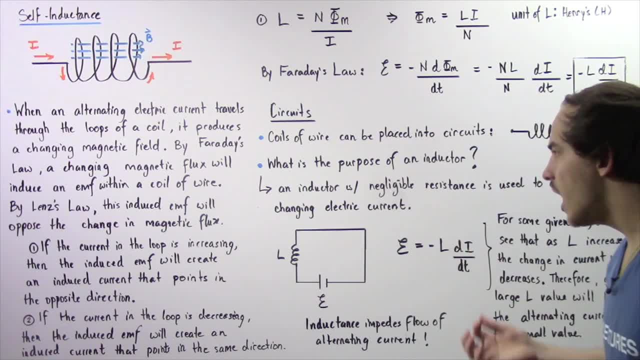 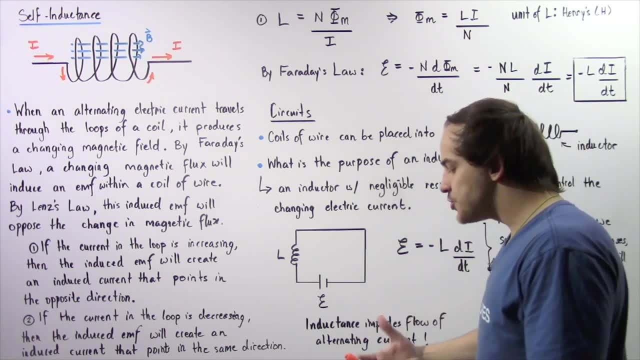 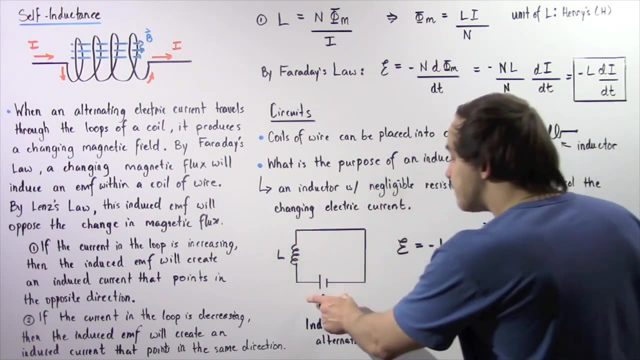 purpose of our inductor. Now an inductor with a negligible resistance is used to essentially control the changing electric current. So let's suppose we have some sort of source of voltage and that voltage is given by the following quantity: Now we know from this equation: 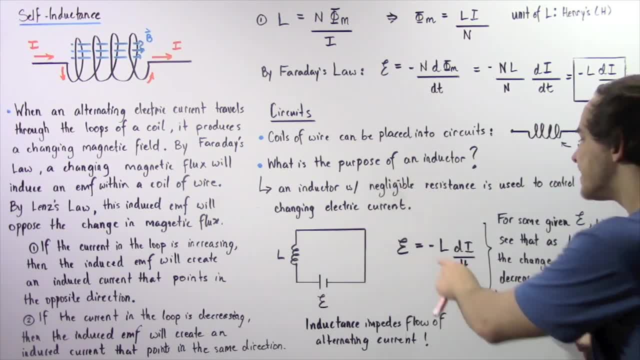 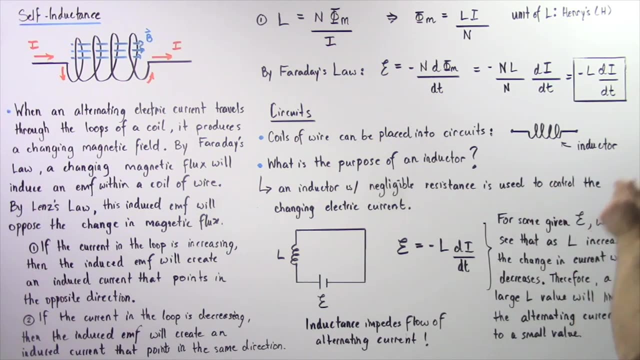 that our induced EMF is equal to negative L multiplied by D, which is equal to negative L divided by DT, where this is simply the rate of change of our electric current with respect to time. Now for some, given quantity of our voltage produced by our voltage source, we see that as L. 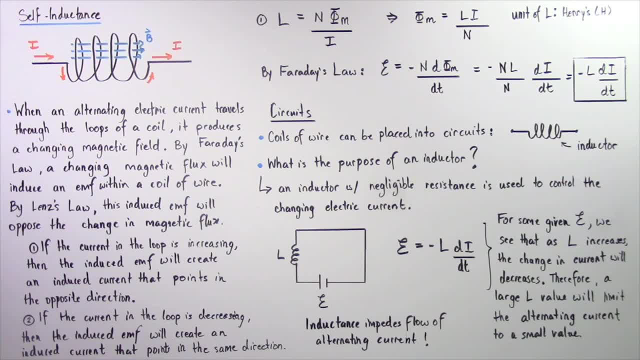 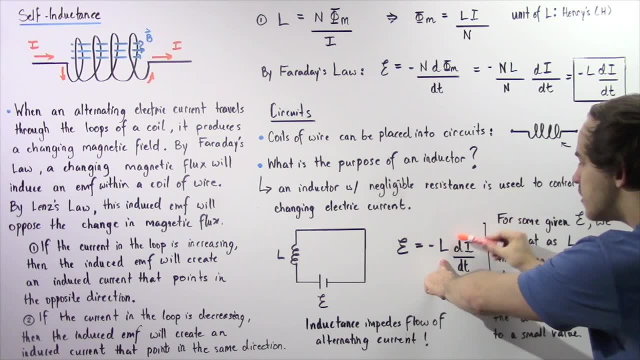 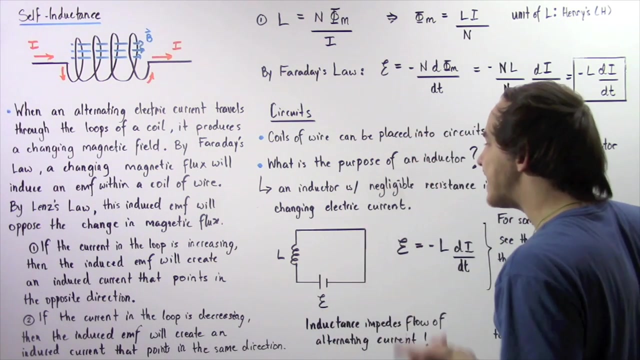 increases, the change in current will decrease. In other words, if this quantity stays constant and we increase the amount of L, this quantity must decrease to compensate this increase, so that this constant remains the same. So if we increase the quantity of inductance within our inductor, that will essentially decrease the rate. 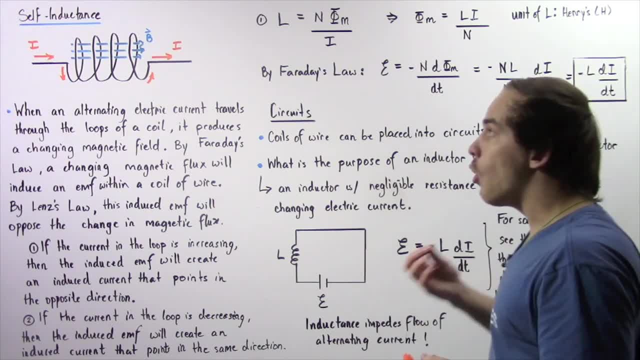 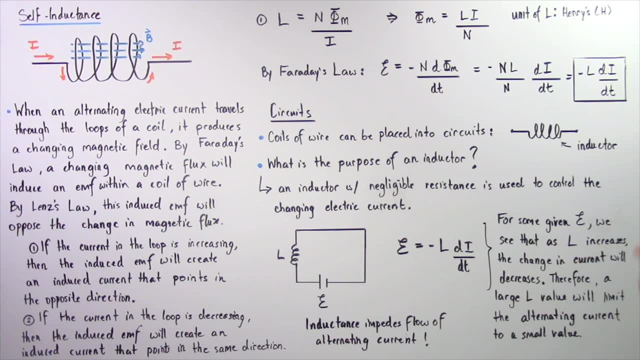 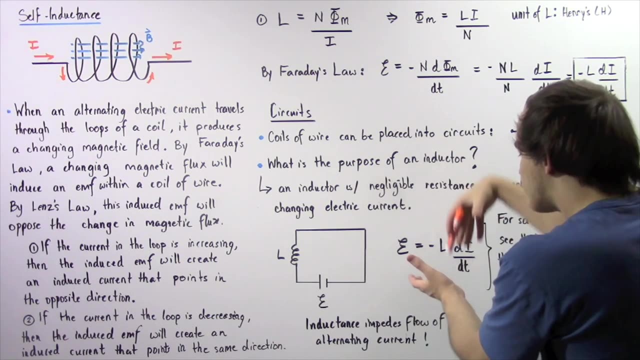 of change of our electric current, and so our alternating current will thereby decrease. So therefore, a large L value will limit the alternating current to a very high value. Likewise, if the L decreases, this rate of change increases and our alternating electric current